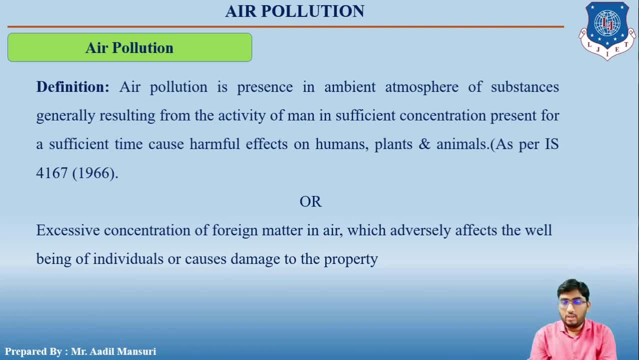 can be considered at micro scale, outdoor air pollution can be considered at mesoscale and air pollution at global level can be considered as macro scale. okay, so now? what do you mean by pollutant? okay, so the? any substance, any substance present in the environment in harmful concentration which adversely 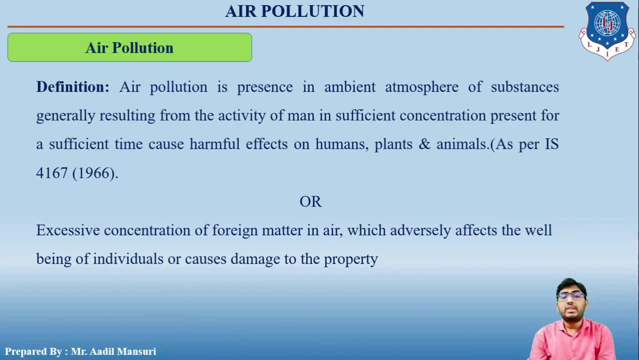 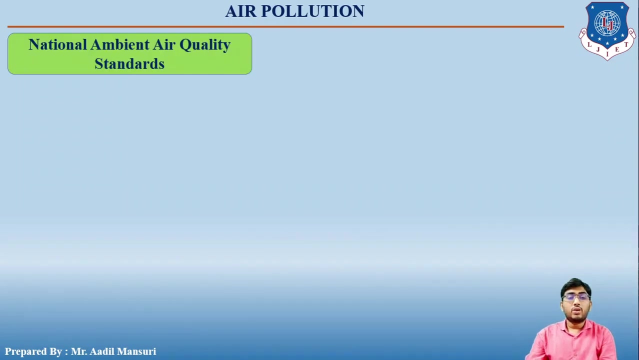 alter the environment by damaging the growth rate of a species, by interfering with the food chains, which is toxic and affects the health, comfort and property, is considered as a pollutant okay, or the particles which cause pollution can be deemed as a pollutant okay. so now so let us talk. 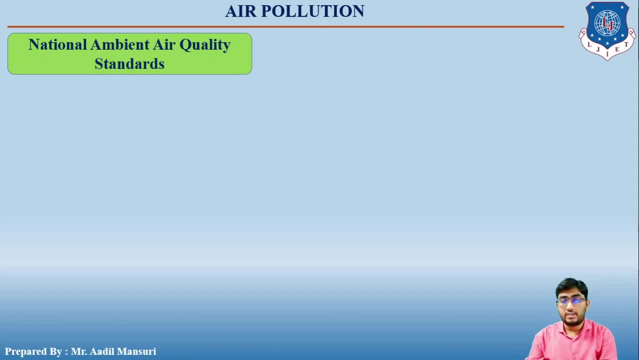 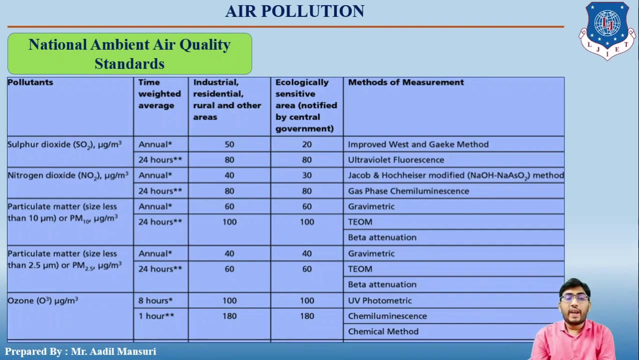 about national ambient air quality standards. so this is a table showing which are the different pollutants, right, when time weighted average: industrial, residential or rural and other areas. right, then, ecologically sensitive areas and made methods of measurement. okay, so these are the different limits, right? so industrial, residential, rural area is also given an 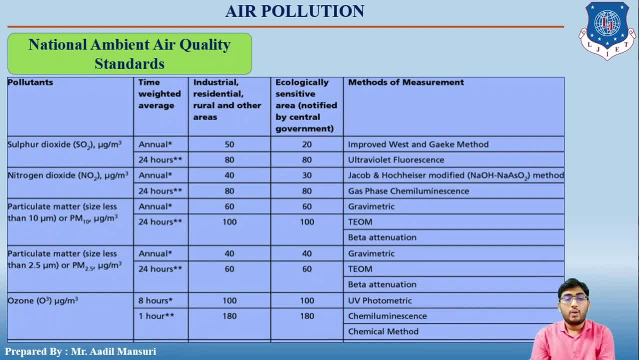 ecological sensor sensitive area is also given. okay, now, here they have written a number that there are different pollutants, right? so first one is the sulfur dioxide, SO2, which is in microgram per meter cube, right. then it is nitrogen dioxide, then it is particulate matter which are of the size less than 10 micrometer, right, or which is known as PM10. 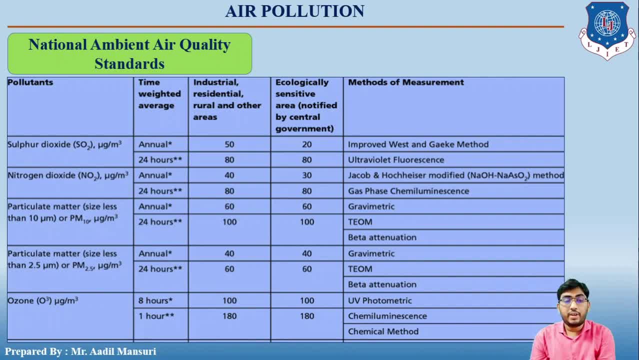 right, and the concentration is in microgram per meter cube, fine, then PM 2.5 and ozone, right? so this is the annual weighted average, or time weighted average means it is the time when it is calculated, right? so there are different times, so one is annual time, then there is 24 hours of time, then 8 hours. 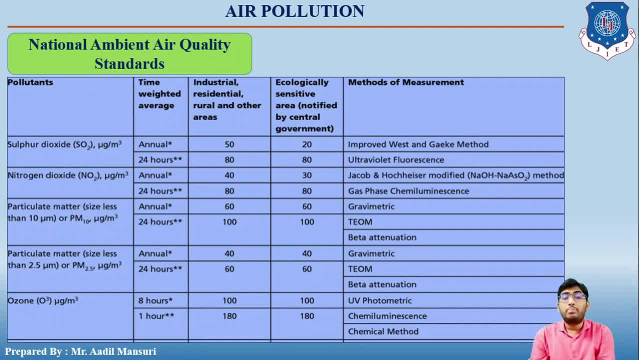 then 1 hours. okay, so what does this annual mean, right? so annual means that- and it is the annual arithmetic mean of minimum hundred and four measurements which are taken in a year at a particular site, right, and which are taken twice a week and at a 24 hourly intervals. okay, so that is known as annual reading. 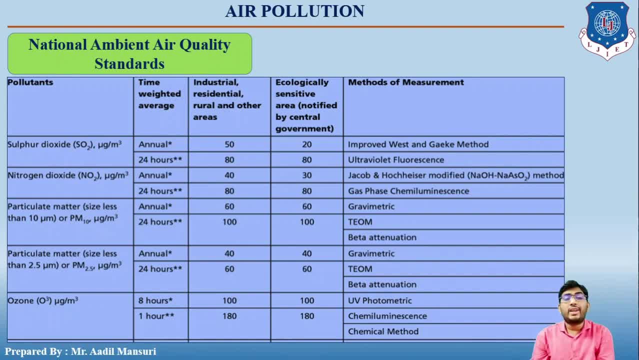 okay, if I talk about 24 hours or 8 hours or 1 hours, then 24 hours, 8 hours or 1 hours, it is the hourly monitored values. that is either it after 24 hours or after 8 hours or after 1 hour. right, it is. 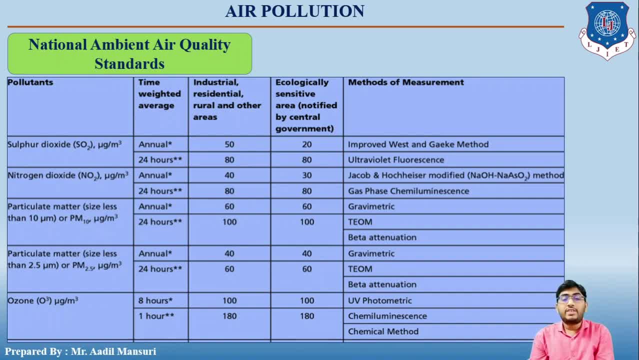 the monitored values which are applicable and shall be compiled with 90, 98 percent of the time in a year right and two percent of the time they may exceed the limit, but not on the two consecutive days of monitoring right clear. so, uh, different values are given for industrial residential. 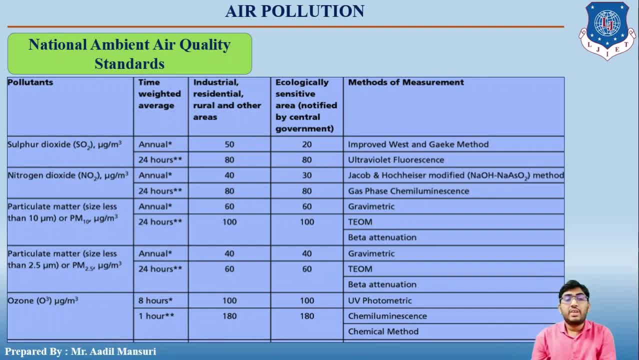 ruler areas, that is, SO2. if you measured annually, it should be uh around 15 right, and for ecologically sensitive areas it should be 20, and different methods of measurement is also given. if you like measure at 24 hours interval, it should be 80, and for ecologically 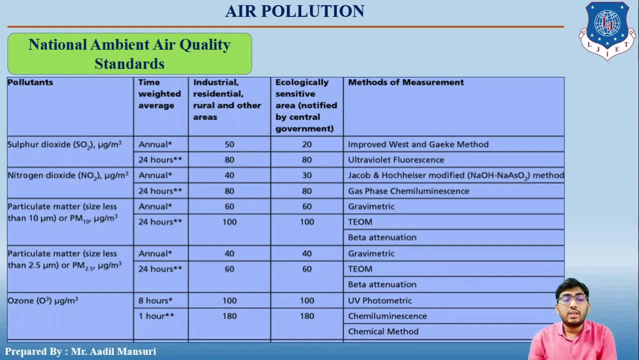 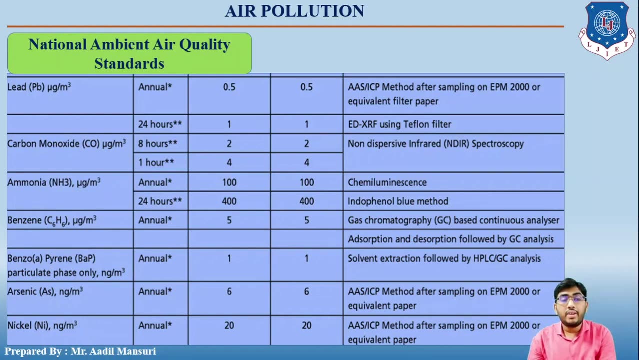 sensitive areas should be also 80, okay. so similarly it is for nitrogen dioxide, PM 2.5, PM 10, ozone- okay. then comes another uh kinds of pollutants, that is lead, okay. PB, uh. so annual value 0.5 and 0.5 and 24 hour values one and one. okay, then there. 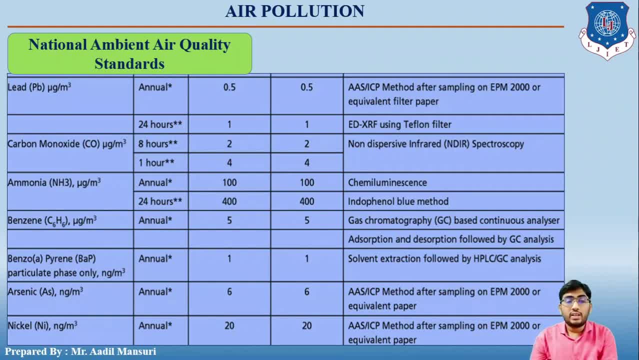 is carbon monoxide, right then ammonia, NH3, benzene, C6, H6. right then benzopyrene, particulate phase only. right then arsenic and nickel. so these are the different pollutants and different values for industrial, industrial areas or ecologically sensitive areas right, which are measured either. 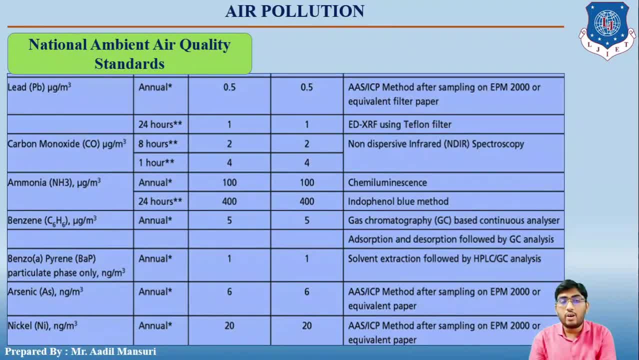 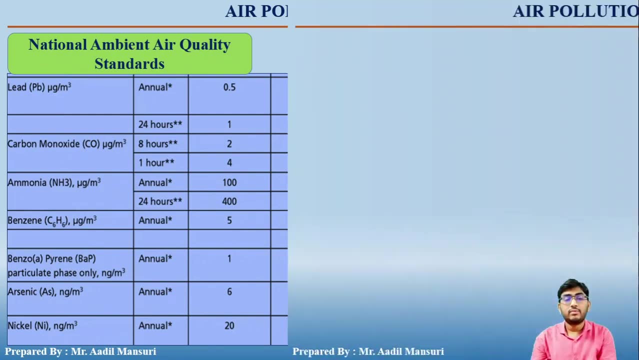 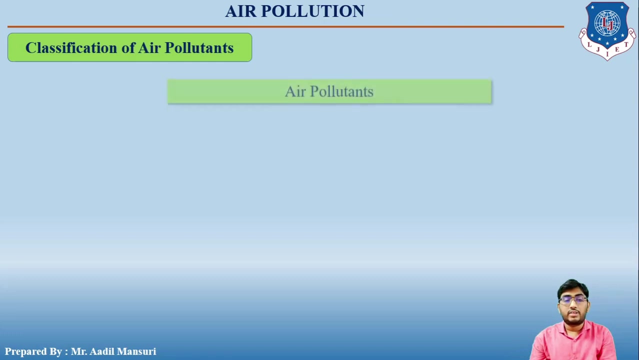 annually or 24 hourly, or eight hourly, or one hourly. okay, so this is the table for a national ambient air quality standards, which is provided by CPCB, that, that is, central pollution control board. okay, so let us move towards the next topic, that is, the classification of air pollutants. 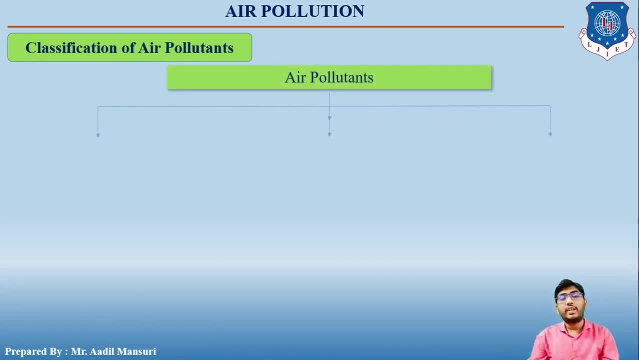 so air pollutants are classified mainly into three types. that is first. one is based on the origin, then it is based on the states of matter and it is based on the presence in environment. okay, so, talking about based on origin, there are primary and secondary pollutants. based on states of matter- there are gaseous and particulate matters- and based on presence in 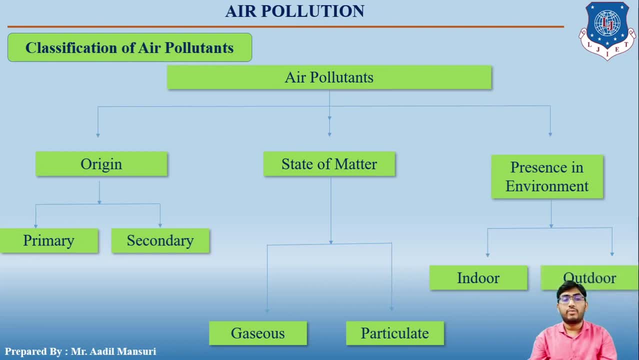 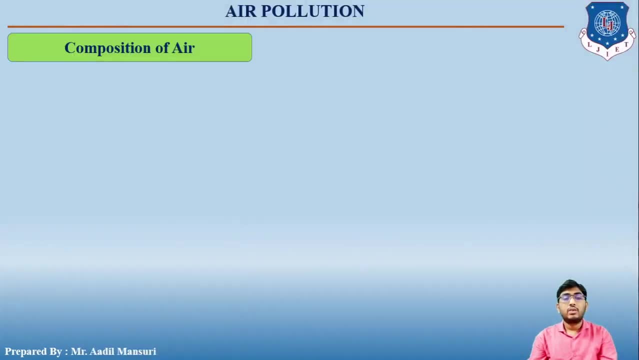 environment. there are indoor and outdoor, okay, so let us have a look at each of them one by one. so before that, let us complete the composition of air. okay, so composition of air: as you can see in the figure right, 78.08 percent is the nitrogen gas, right, it is concentration by. 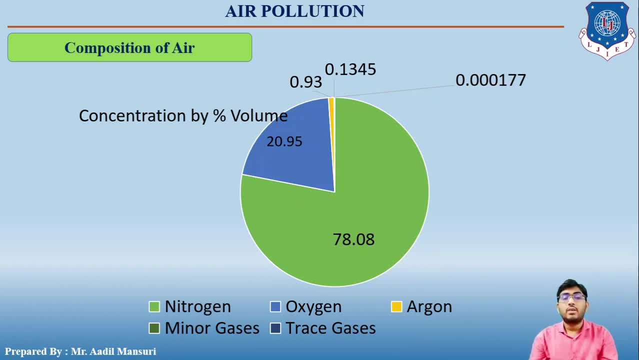 weight concentration by percentage volume. okay, then oxygen: 20.95, then it is the argon nine, point sorry, 0.93 percent. then minor gases and trace gases, that is 0.1345, and point triple zero, one, double seven. okay, so talking about which are the different minor gases, it includes water vapors, that. 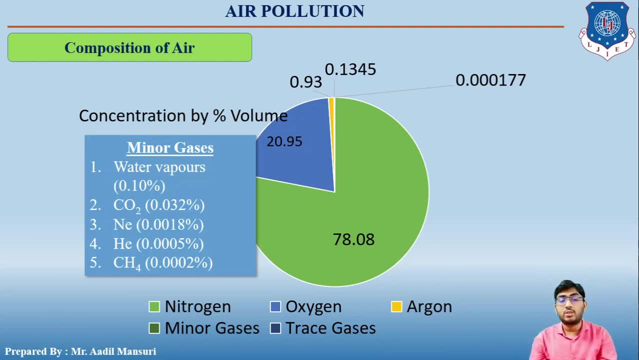 is point one percent. carbon dioxide, 0.032 percent. neon- point double zero, one. eight percent. helium, point triple zero, five percent. and methane, that is point triple zero, two percent. okay, then, talking about the trace gases, which includes krypton, which is in uh, point zero, point triple zero one percent nitrous oxide. 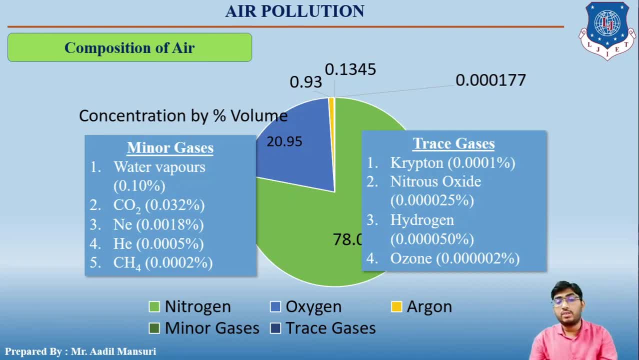 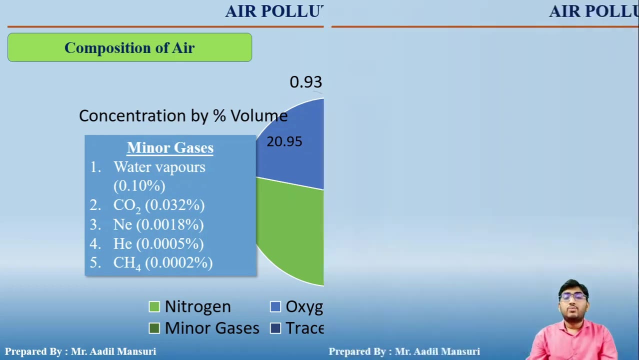 which is point double zero, double zero, two, five percent. hydrogen: point double zero, double zero, five, zero percent. and ozone, point double zero, triple zero, two percent. okay, so this is the composition of air. right now, let us move towards the next topic, that is, the primary air pollutants. 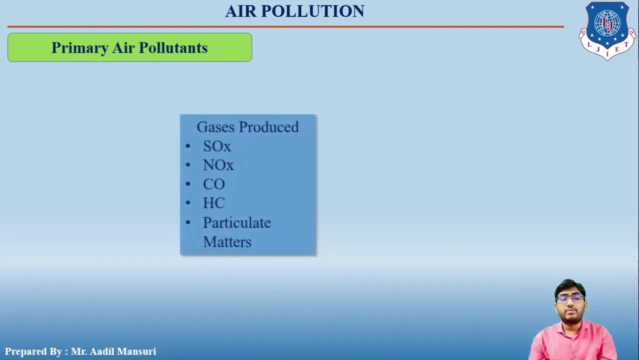 so which are the different primary air pollutants which are present in the atmosphere? so these are the different gases which are produced and which includes oxides of sulfur, oxides of nitrogen, that is, sox and nox, then carbon monoxide, hydrocarbon and particulate metals. okay, so, talking about the different sources of this primary air pollutant, it is 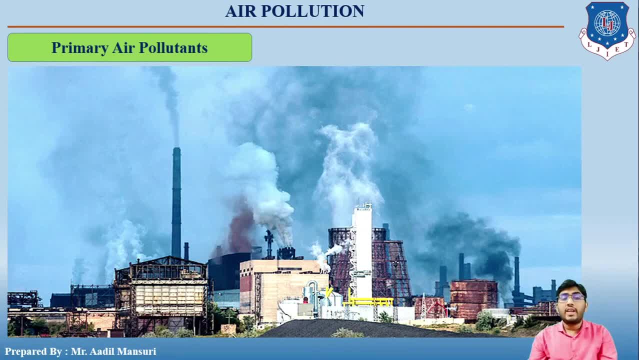 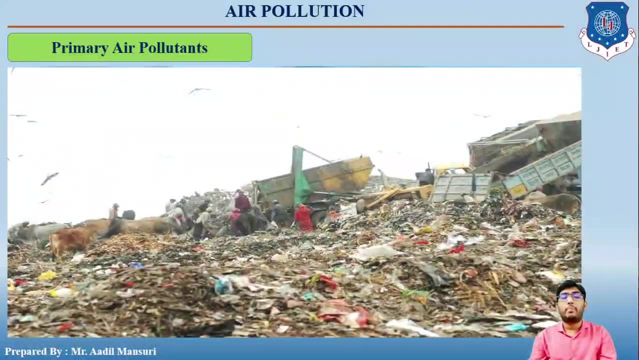 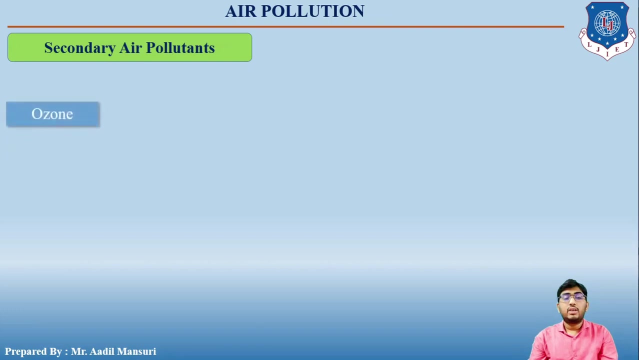 the vehicular emission. then it is the industrial industrial gases or industrial exhaust right and solid waste dumping clear. so these are the different sources of primary air pollutants. let us move ahead talking about the secondary air pollutants. the first one is the ozone, that is o3 molecule, then sulfur trioxide, that is so3. 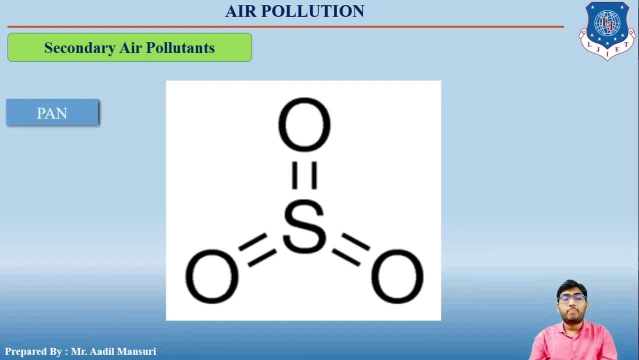 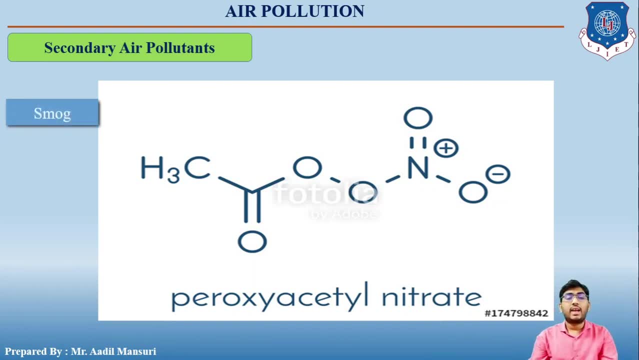 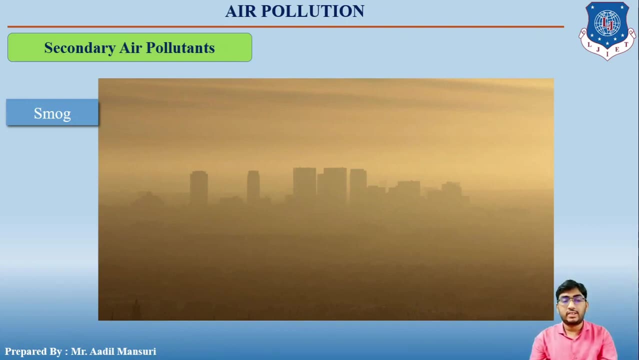 right, then it is pan, that is peroxy acetyl nitrate, right. and the last one is the smog. okay, so these are the different sources of primary air pollutants. let us move ahead. these are different secondary air pollutants. let us now move ahead with the next one, that. 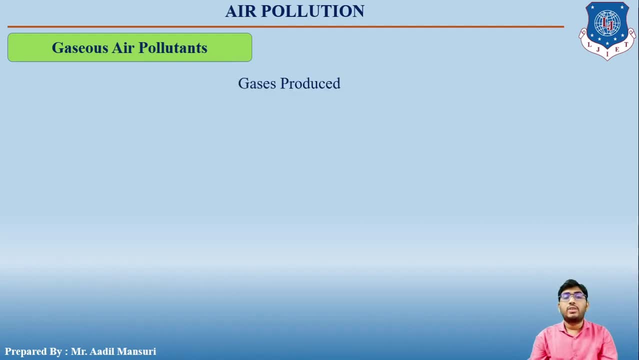 is the gaseous air pollutants. so different gases which are produced are oxides of sulfur, oxides of nitrogen, carbon monoxide, carbon dioxide, hydrocarbon and photochemical oxidants. okay, so these are considered as gaseous air pollutants, then particular air pollutants. so first one is the aerosol, then dust, then fumes, then smoke, then mist, fog, fly, ash, soot. 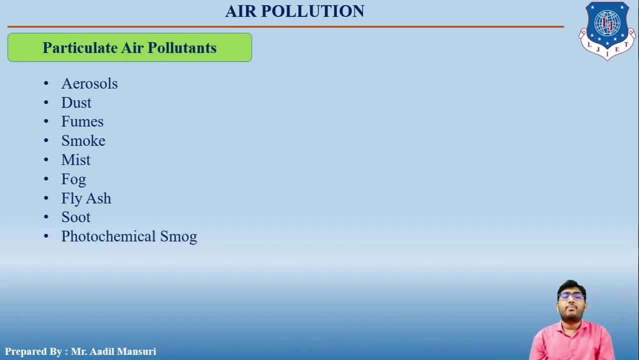 photochemical smog? okay, so what do you mean by a particulate? okay, so particulates are finely divided, airborne solid and liquid particles which remain in the air in the form of gaseous air pollutants, and they remain for a very long time in air in suspension. okay, depending. 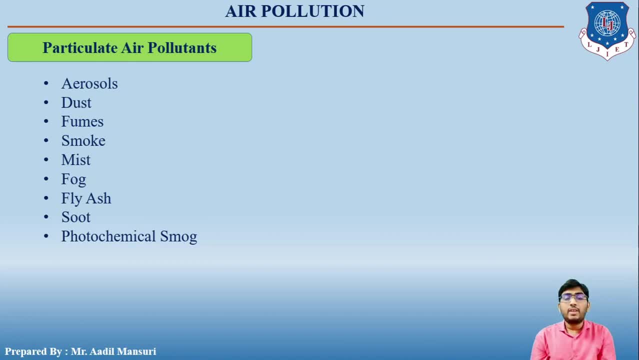 upon their size and mode of formation, particulate air pollutants are classified as shown on the screen. okay, so talking about what do you mean by aerosols? so these are airborne suspension of solid or liquid particles which are smaller than 1 mm size. right, which include dust smoke. fumes, mist and so on. okay, so these are the air pollutants that are classified as particulate as shown on the screen. okay, so, talking about what do you mean by aerosols? so these are airborne fumes, mist and so on. okay, so these are the air pollutants that are classified as particulate. 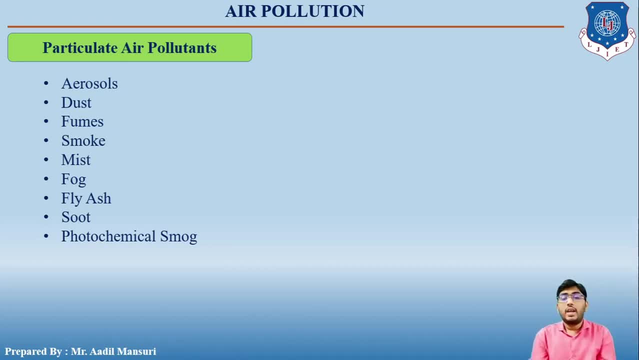 okay, so these are the air pollutants that are classified as particulate. okay, so, talking about dust particles, it consists of small solid particles of 1 to 200 micrometer size and are generated by material crushing or grinding or blasting. they remain in suspension, but finally settle. 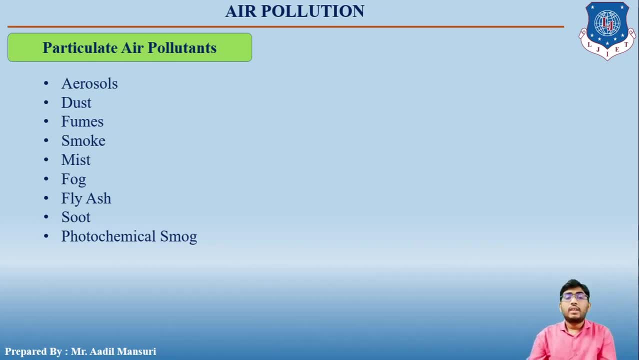 under the effect of gravity. then, talking about fumes, they are fine solid particles of size around 0.1 to 1 micrometer which are formed by condensation of vapours of solid metal. they are odourless vapours which may or may not be visible. okay, then talking about smoke. 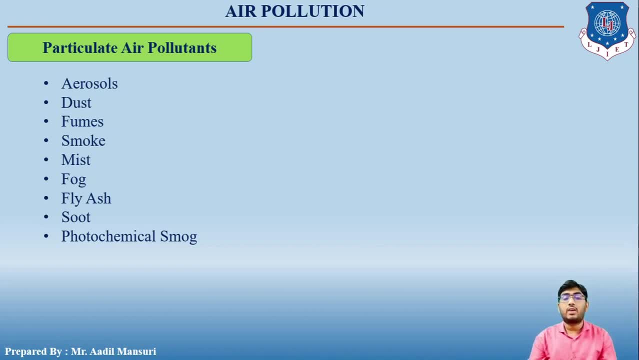 they are also fine, solid particles of size around 0.1 to 1 micrometer, which are formed by incomplete combustion of organic matter, like coke and wood. okay, this is dominated by organic mix, which causes air canal in circulation because it is used for carbon neutral production. 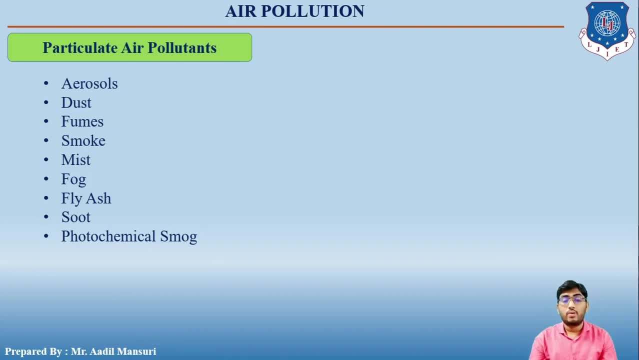 of these, or spores, sleep insectада configures as a 설�kehr, and the ones which are suspended because the corker temperature is between 16 and seven degrees Celcius, degrees which makes wax going even bigger than a tiny spot. Now, depending upon the nature of the material burnt, smoke may have different odors. okay, 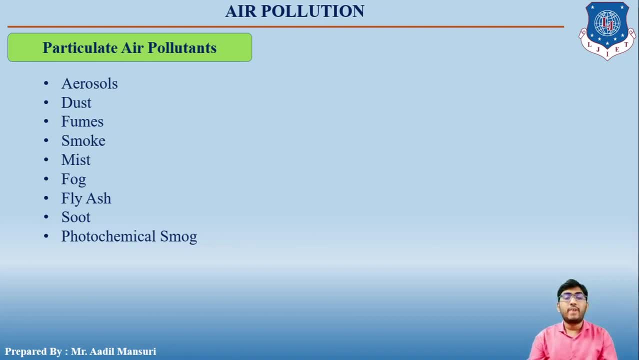 Then let us talk about mist. So what do we mean by mist? So it consists of liquid droplets of size around 0.1 to 10 micrometers and formed by the condensation of vapors in the atmosphere. right? 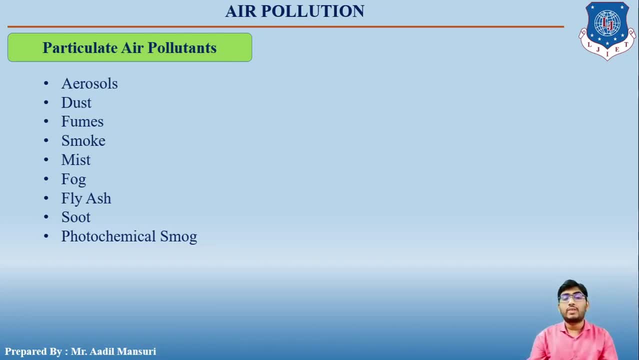 Then fog. So if the above said mist is made up of droplets at high concentration so as to obscure vision, then mist is called fog. okay, Then fly ash. These are inorganic substances released after the burning of organic particles from coal. 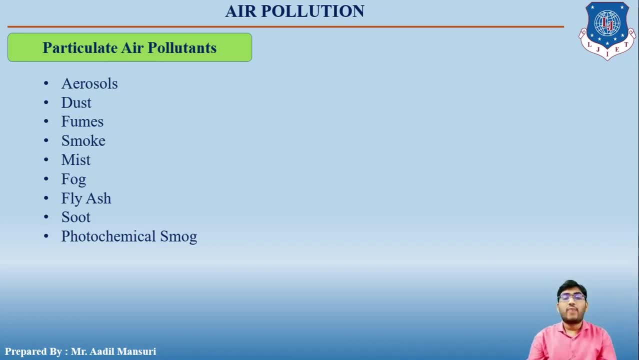 or wood? okay, These are finely divided, non-combustible light particles present in the air, So they are called carbon gases. Talking about soot, these are carbon particles impregnated with tar and released by the incomplete combustion of carbonaceous material. okay, 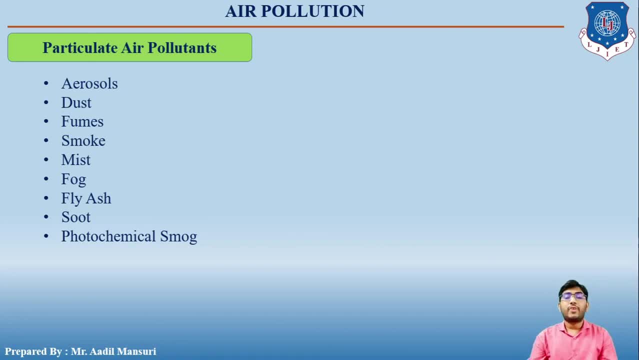 And last, talking about photochemical smoke: atmospheric pollution formed by chemical reaction among hydrocarbons, ozone and other pollutants in the presence of carbon. So these are carbon particles impregnated with tar and released by the incomplete combustion of carbonaceous material. 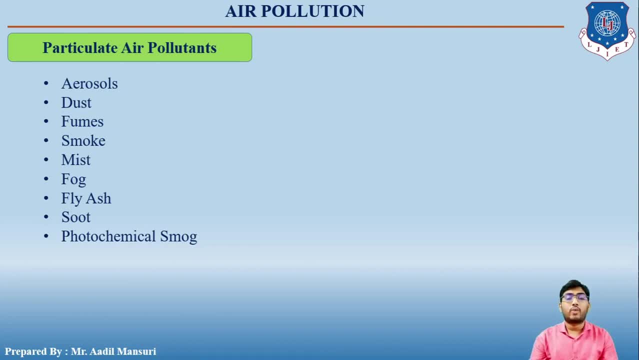 This toxic carbon is called carbon monoxide. The presence of sun light in the presence of carbon monoxide is referred to as photochemical smog. okay, So let me show you the different photographs. So the first one is the dust one. 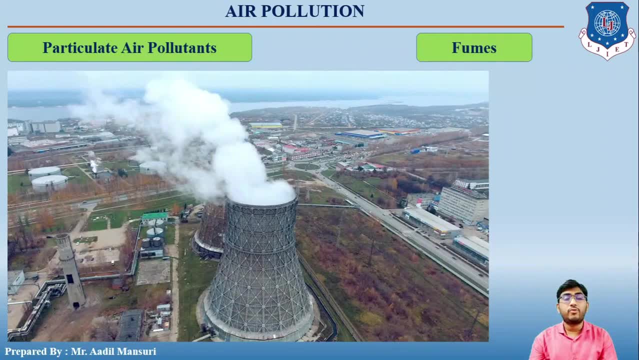 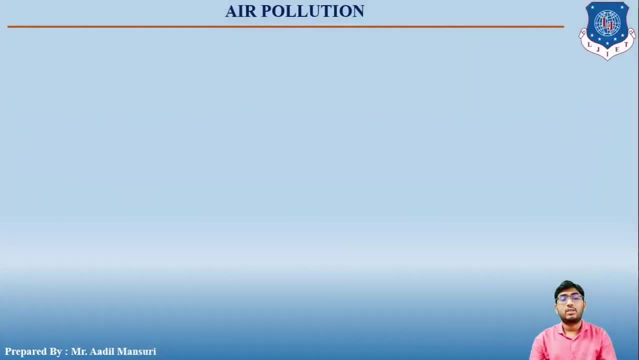 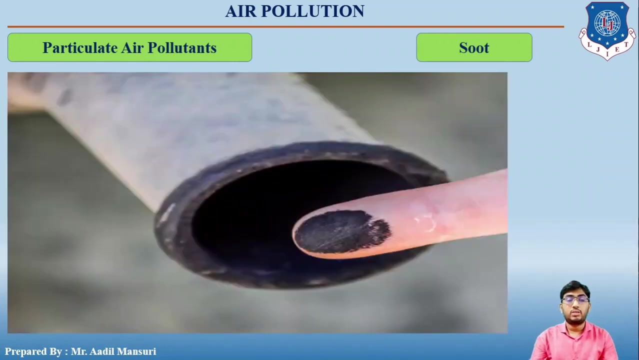 Then it is fumes. You can see the fumes getting out or coming out from the chimneys of thermal power plant. Then it is the smoke, based on different particles. First one is the liquid smoke, which are burnt, then it is mist, then it is fog, then it is suit- okay, then it is. 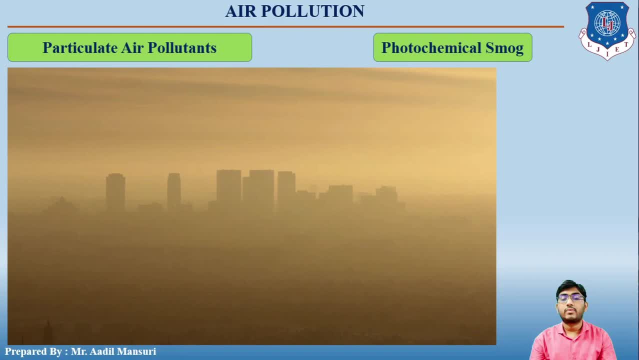 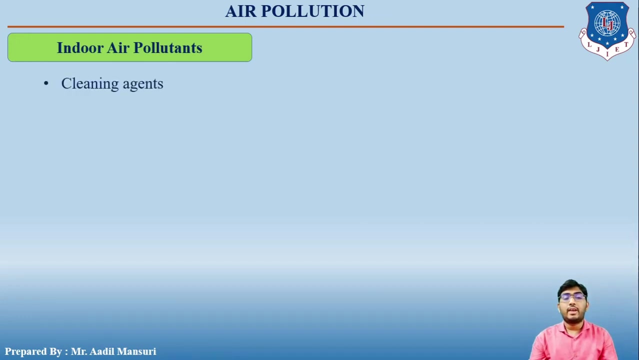 the photochemical smog. okay, so, my dear students, this is the complete classification of particulate air pollutants. let us now move ahead with the indoor air pollutants. so different chemical agents, pesticides, cigarette smoke, microbes like bacteria, virus and fungi, mosquito repellents, paints loose and varnishes. okay then, gases from stoves.